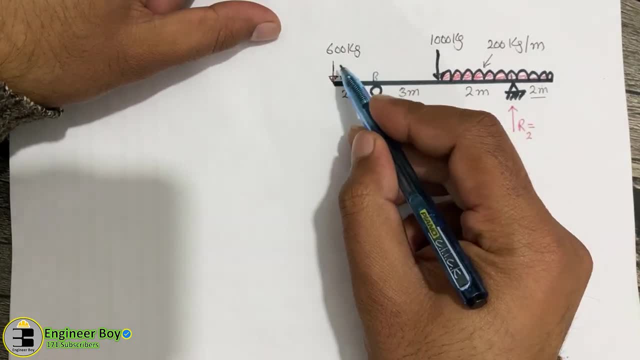 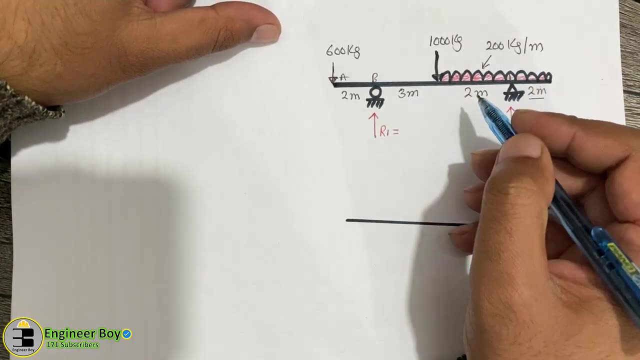 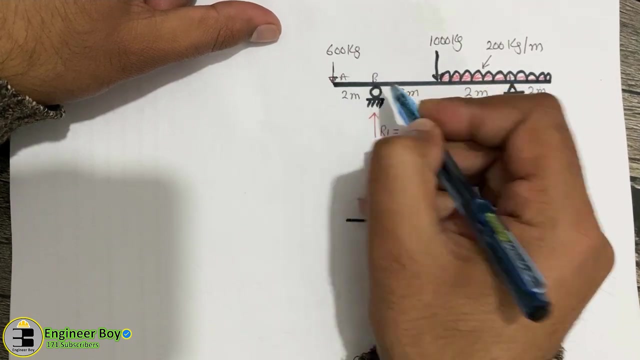 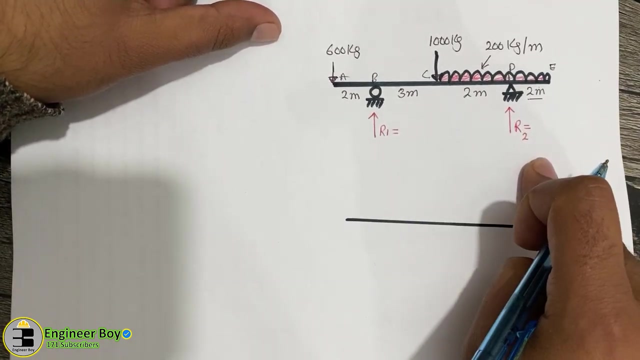 Okay. so if you remember, previously on engineer boy, we have determined the support reactions of a single overhanging beam. This time we got a double overhanging beam, Okay. so in this video we will be determining reaction one and reaction two. Okay, let's say, this is point A, this is B, this one C, this one D, and there we got E. So let's just determine R1 and R2.. And for this let me just suppose some equilibrium equations. I'll say the sum of 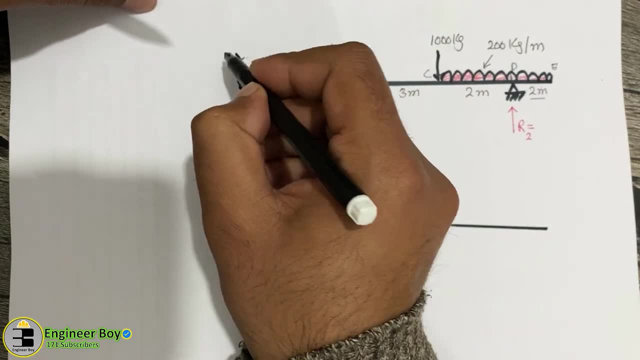 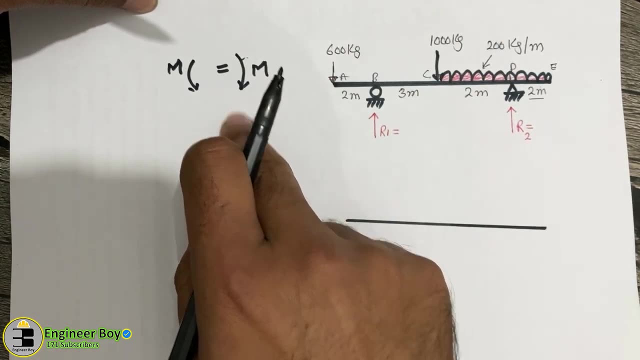 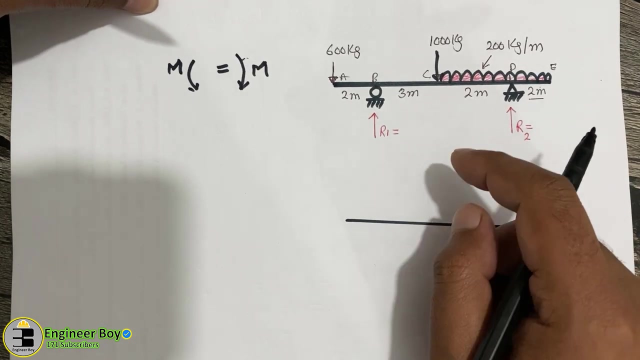 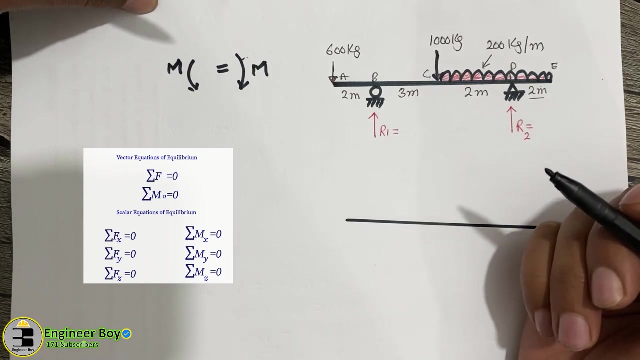 moment, or you can say the clockwise moment, that is going to be equal to the anticlockwise moment. So we suppose these equilibrium equations in order to determine R1 and R2, because this is just a determinate structure and we can analyze this with equilibrium equations. Equilibrium equations are actually the sum of, or you can say: forces in vertical direction must be zero, the summation of forces in horizontal direction must be zero and the summation of moment it. 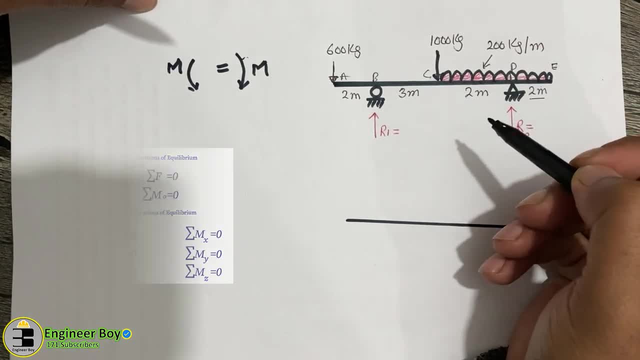 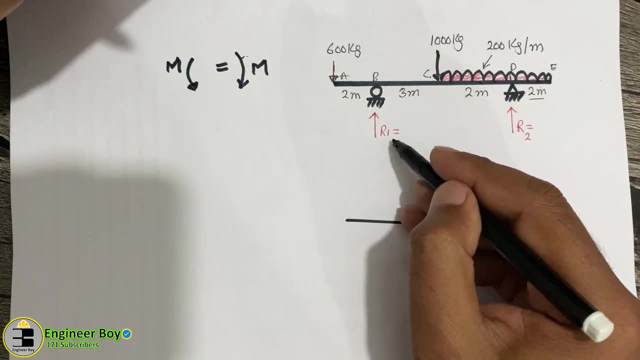 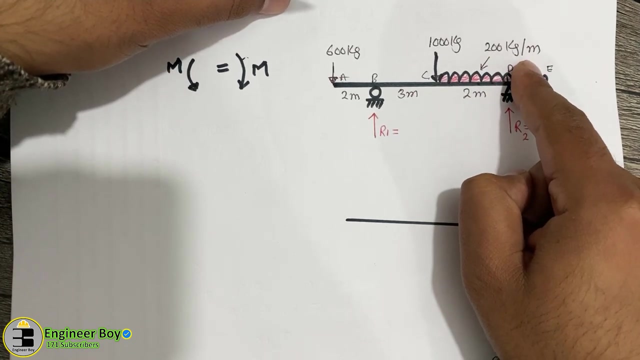 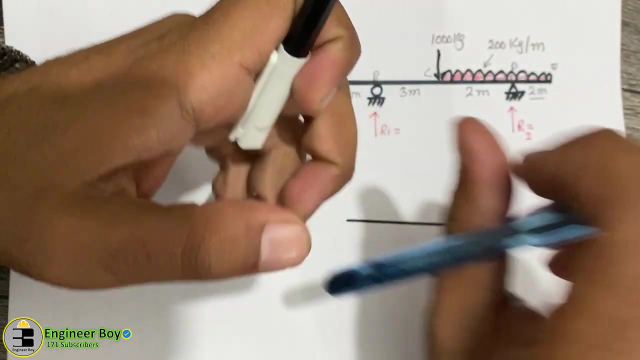 one point. Okay, there can be any point along. the span must be zero. So this time I'm going to say the anticlockwise moment equals the clockwise moment. Okay, to determine R1 and R2.. Now, as you can see, we got UDL, which is 200 kg per meter. So actually, to make it easy, we gonna convert that into a point load. Okay, that's why I have drawn this line. This is, let's say, a beam, And here we got R1.. 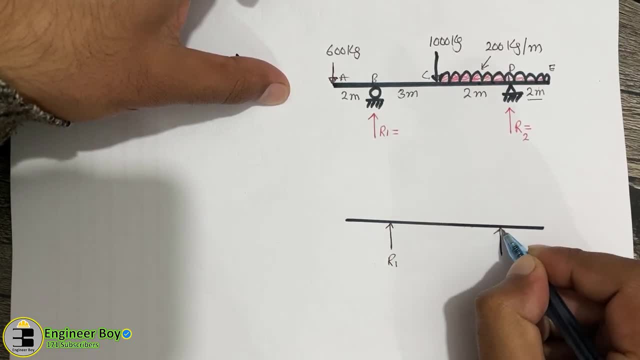 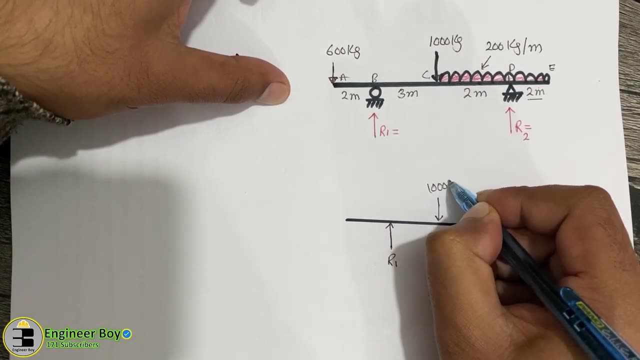 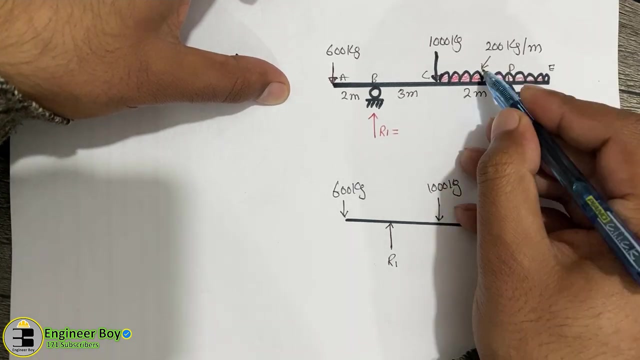 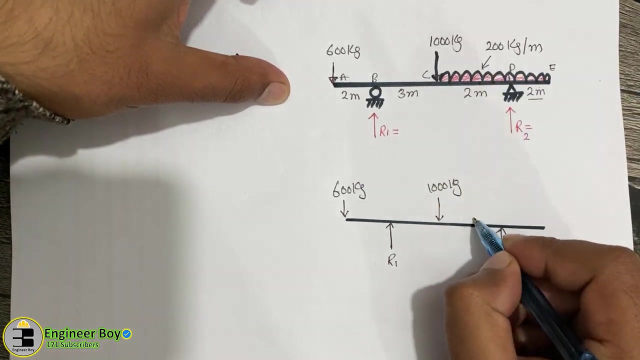 Okay, that is reaction one, And there we got R2, which is reaction two. Okay, And as you can see, at the middle we got 1000 kg. At the left hand side we got 600 kg. Now let's just convert this UDL, As you can see, on two meter span. there we're gonna take a point load over here, Okay, And that is 200 kg, But that is per meter. 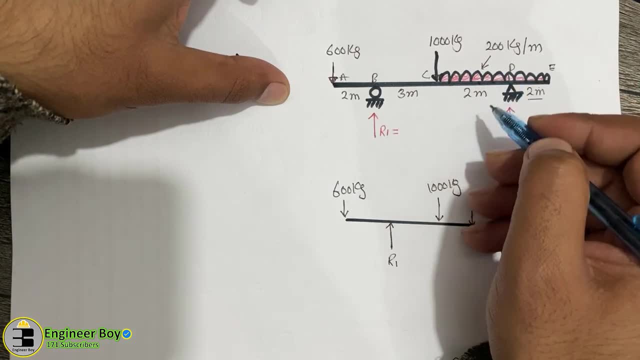 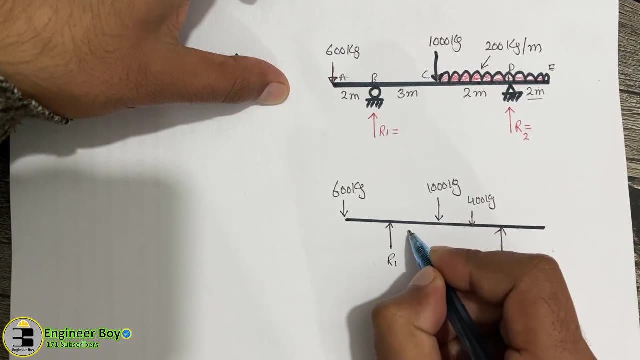 so we're gonna multiply that with two in order to get a point load. so two, twos are, that is four. so i can say: 400 kg is here. that is actually three meter. this one is two meter and here we got that is two meter. so we are gonna, uh, just divide it into two spans, one meter and one meter, and we 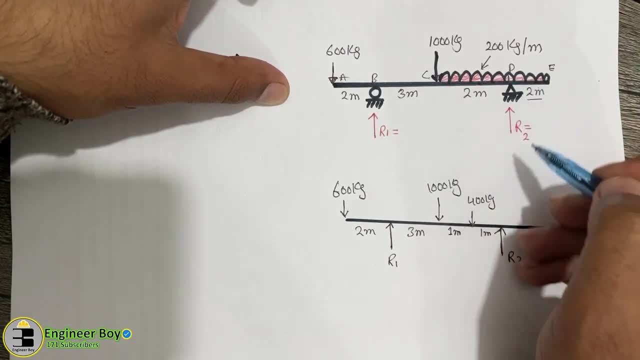 gonna do that, the same thing with this. okay, this we're hanging portion, so that is actually a point load at midpoint, and there we have actually 400 kg, which is actually 200 times this two. okay, so we have just converted that into point load. here we have one meter and there we have one meter. so 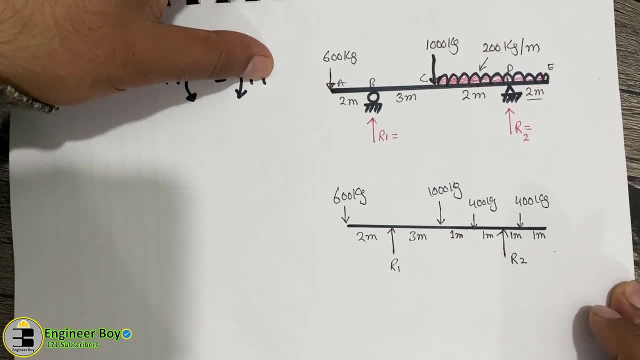 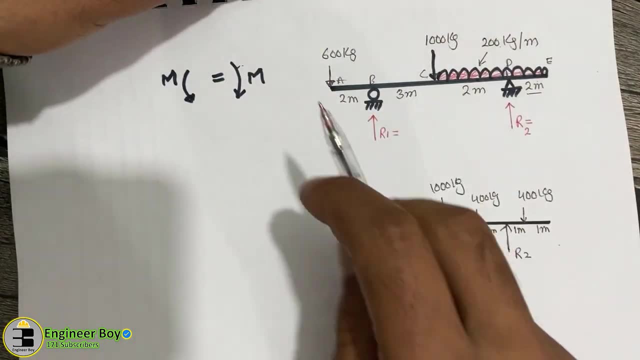 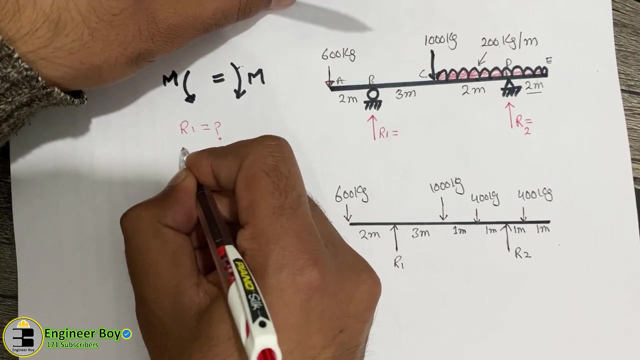 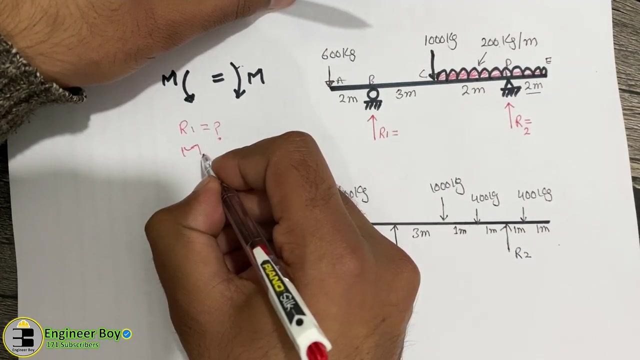 simple, nothing complicated here. okay, all right, now let's just determine the support reactions and for this suppose approach. as you can see, we got clockwise moment and any clockwise moment. now, in order to determine r1, okay, i'm going to take moment, this moment it, you can say r2, or maybe at point d, okay, so i'm. 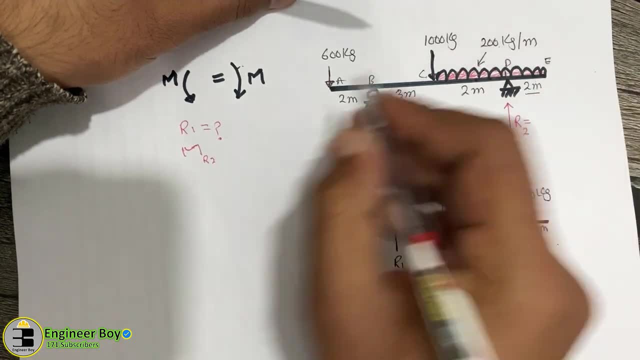 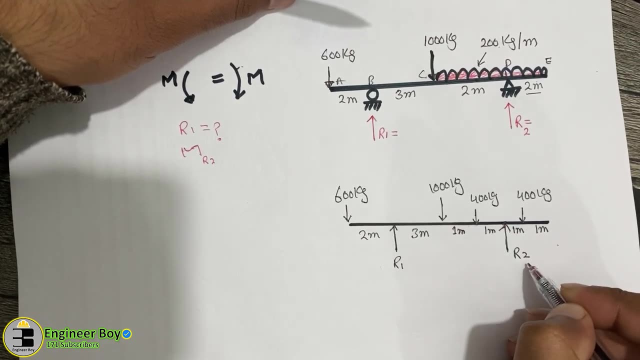 going to take moment at point d or r2. okay, so in order to take moment at point d, reaction 2, as you can see, this force is just downward. okay, that is making the rotation like that toward r2. so that is actually any clock. you can see that. 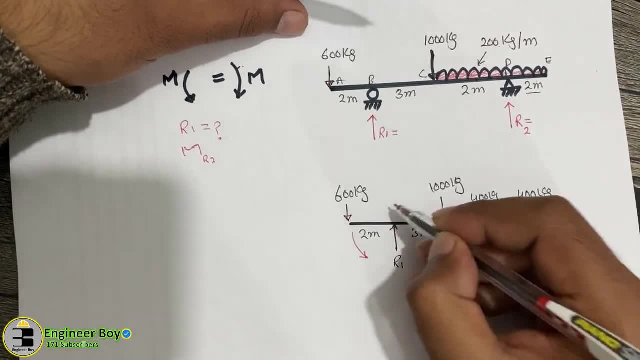 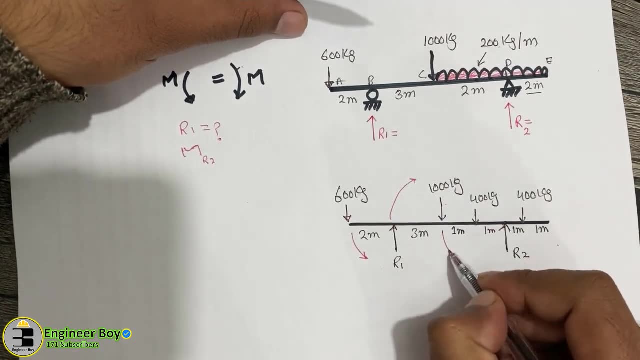 is anti-clock. now this reaction, which is upward and that is just toward r2, so that's just clockwise. you can see that now this force, this is any clock, this one, that is anti-clock, and here 400 kg, that is actually clocked, because that is downward and toward this r2, so that's just clockwise, so that's. 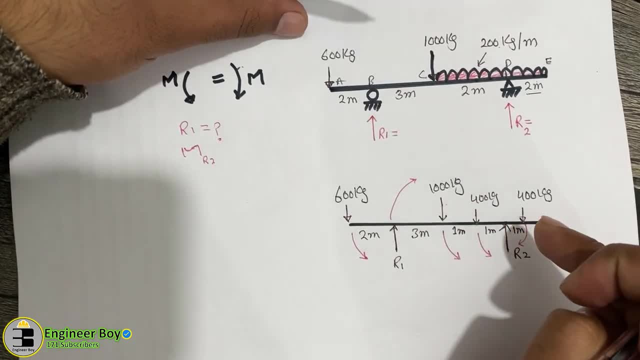 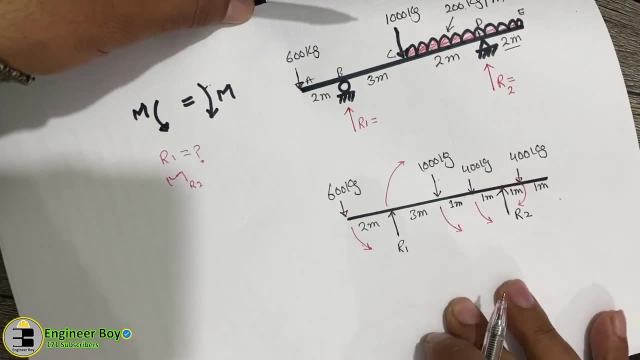 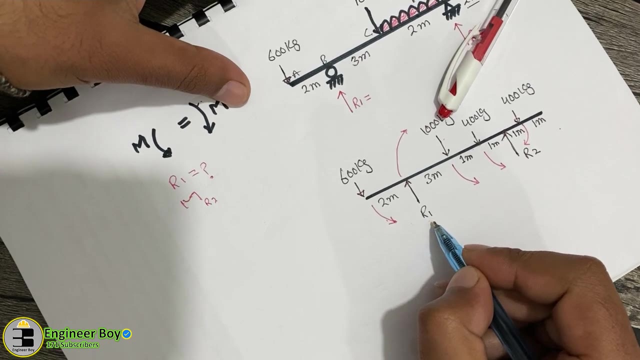 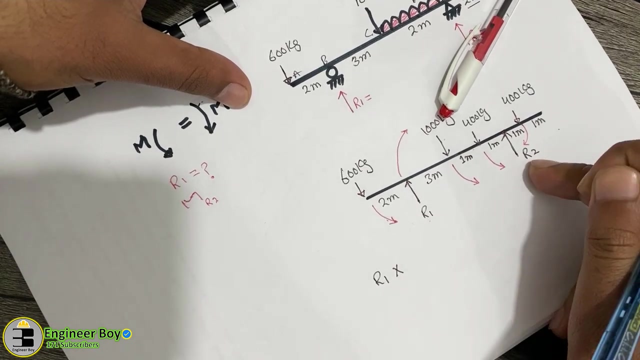 so this time you got two clockwise and actually, when this is clock, when this is, and these three are any clock, okay. so let's just um do some mathematics with this. okay, now let's do it. as you can see, i'm going to determine r1 and that is actually clockwise. okay, so r1 times the distance toward r2. 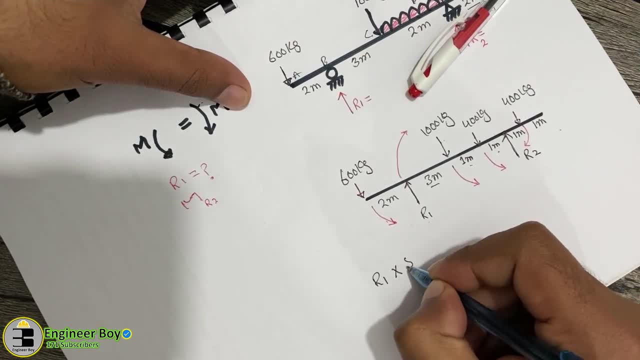 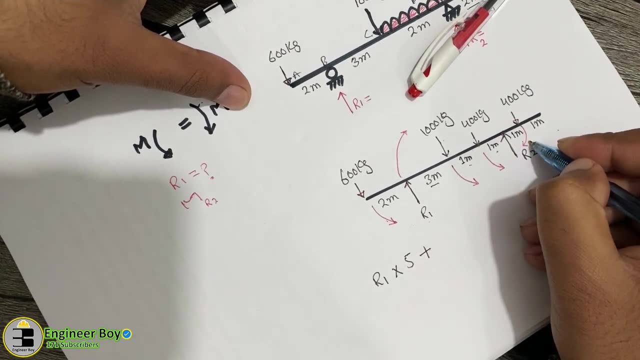 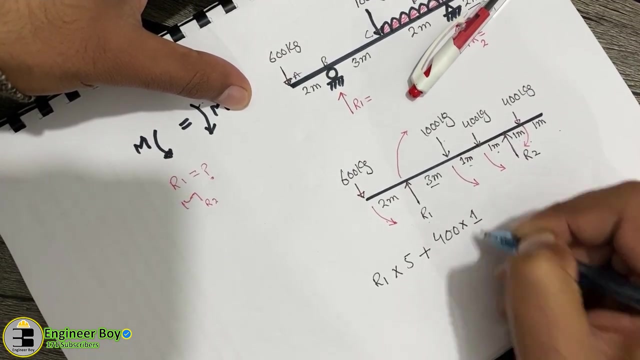 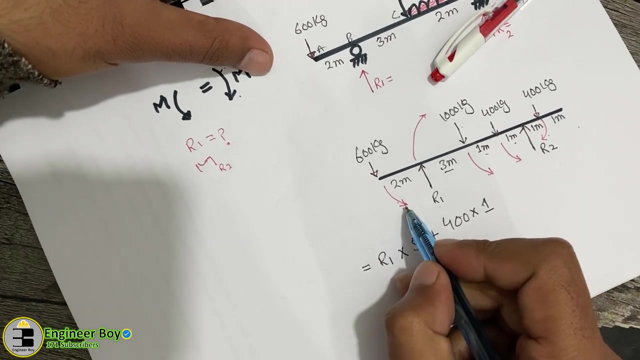 and that is actually three meter, one meter and one meter, that is five. okay, this is clockwise. now another clockwise, that's this one that is actually clockwise, and that is 400 times the distance, which is one meter, toward r2. okay, now this is clockwise. at the left hand side, i'm going to mention any clock. okay, this one is anti-clock, and 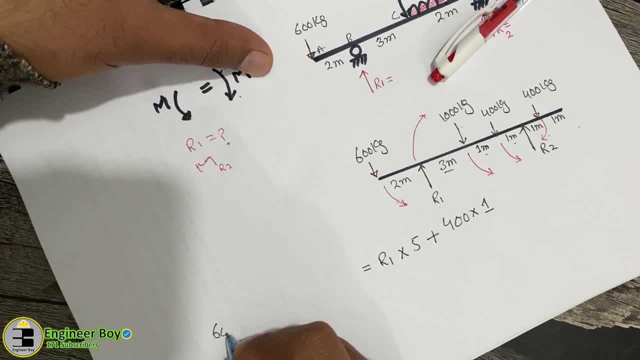 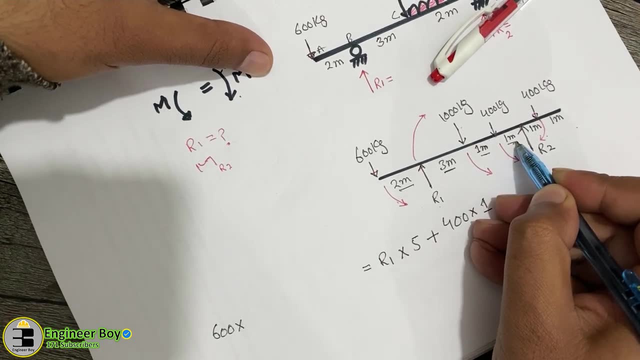 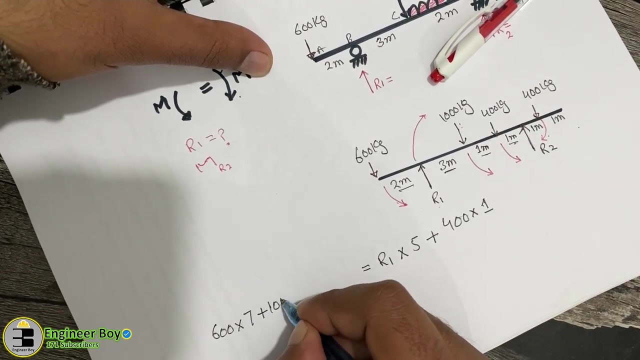 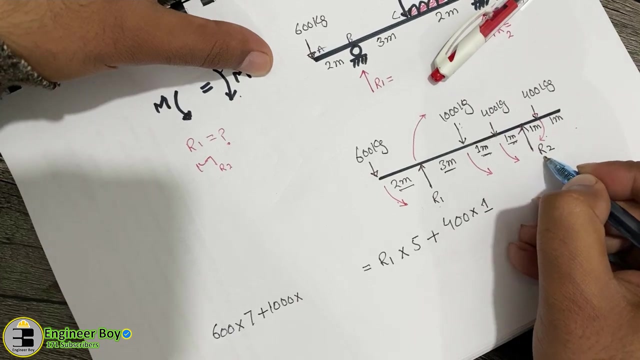 that is actually 600, if you see it, times the distance. this is two, three. that is five, six and seven. so times seven plus 1000, that is anti clock times distance. that is one meter and two, actually one. one that is just two meter toward r2, plus we have one remaining. 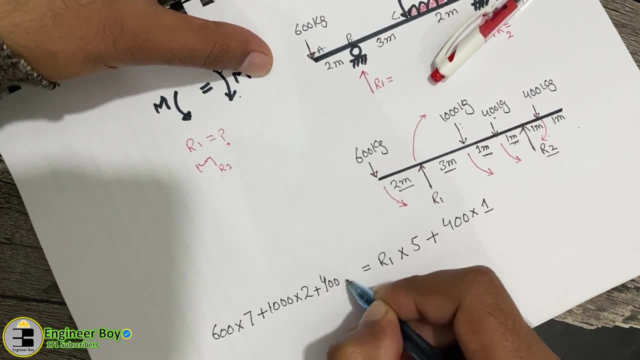 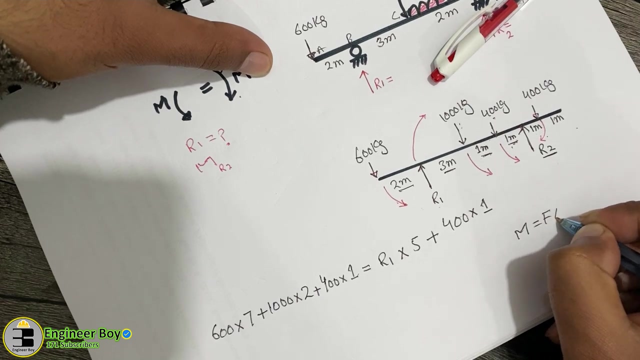 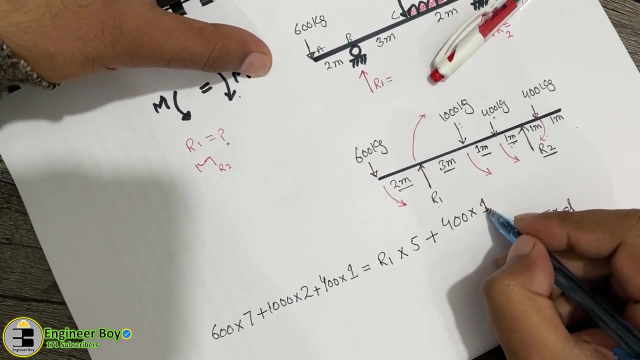 that is, 400 times distance till r2. that is actually one. why we are taking actually the distance is because moment, moment is actually the force times the distance, the perpendicular distance till the point. okay, that's why we are taking the distance. now let's just simplify it. 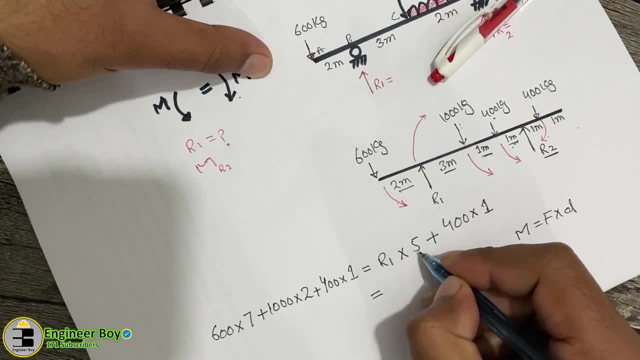 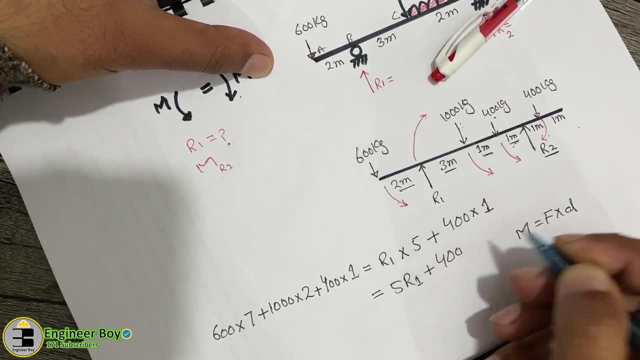 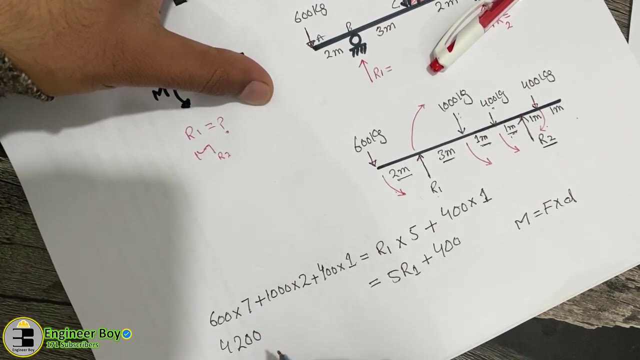 so we can determine r1. okay, here we got five r1 plus for ones are that is actually 400, six, sevens are that is 4200. this is actually two thousand and four hundred. okay, now, at these three we can get actually 6600 and we can just. 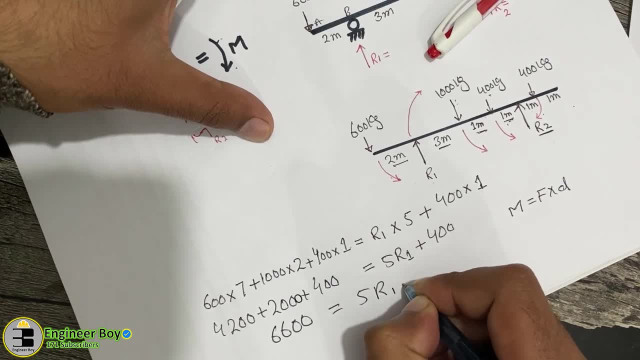 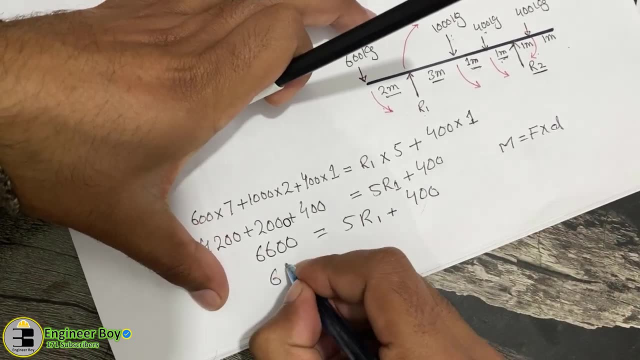 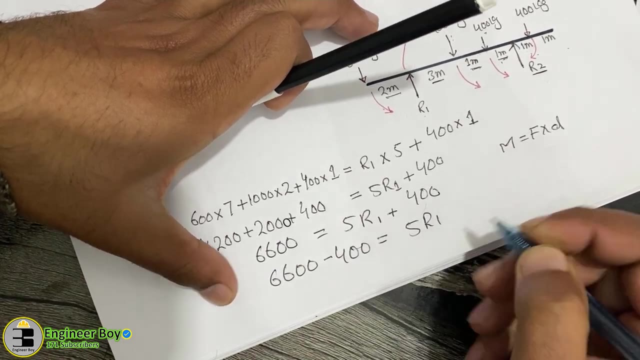 okay, let's just write data again, so there is no confusion again. now just bring that to the another side of the equation. we going to subtract four, all right, so we get actually 5 r1. now we don't need five r1, we actually need r1. so let's divide both. 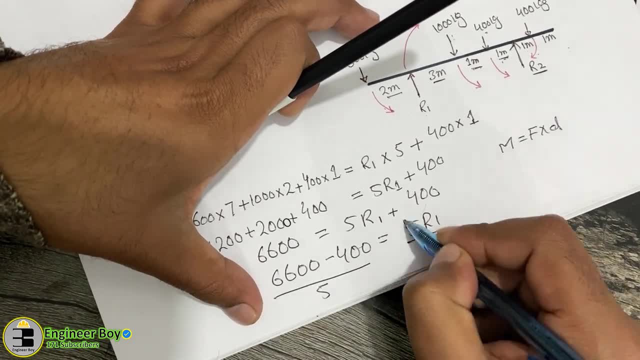 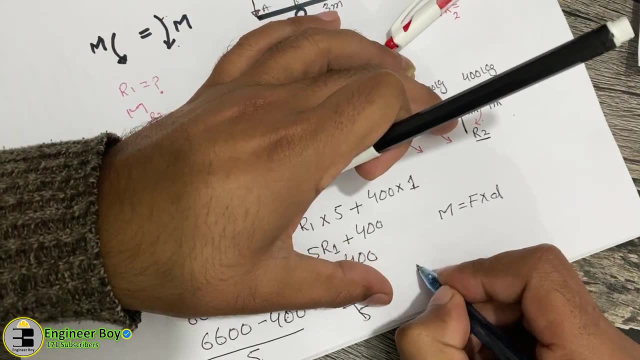 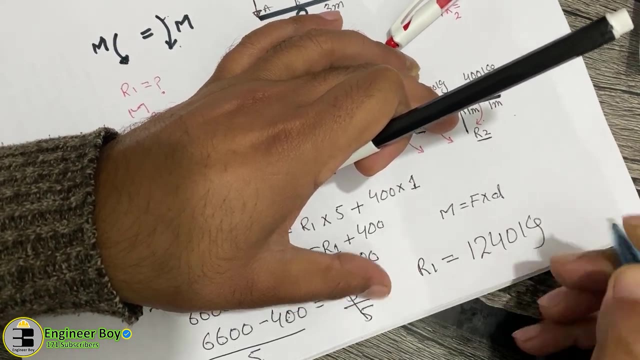 sides by a five, five actually. okay, so these two cross each other. now just do, let's subt·re this one and divide it by five, so we get each other the last in. hey, that's затar r1 and it is, if I'm not wrong, 1240 kg. okay, so we have just determined r1 and 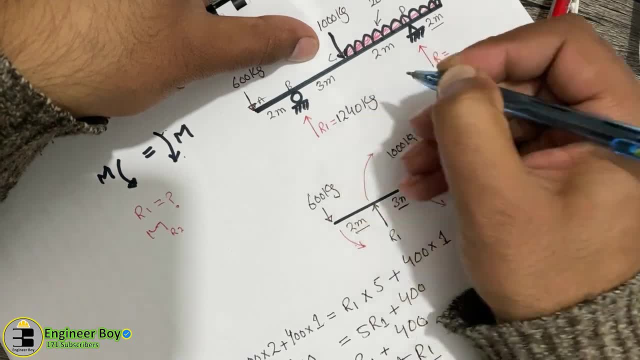 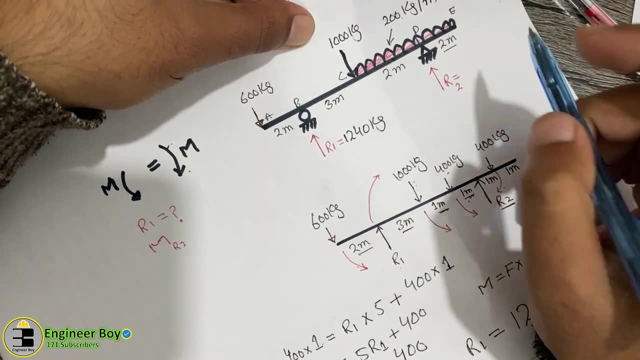 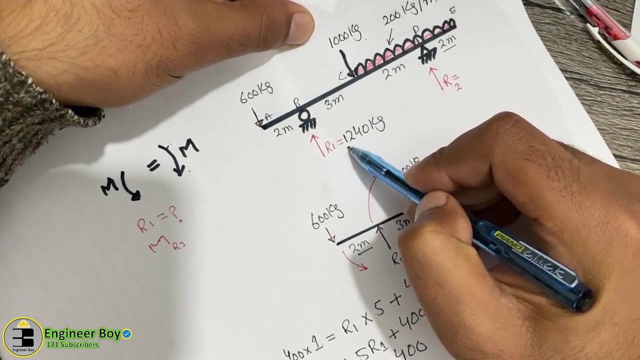 it is 1240 kg. so simple, nothing complicated here. okay, now let's just determine r2, and there's gonna be so simple. we are going to subtract r1 from the total load, because r1 is already taken right, it is already been supported and the remaining force is going to be supported by r2. let's just